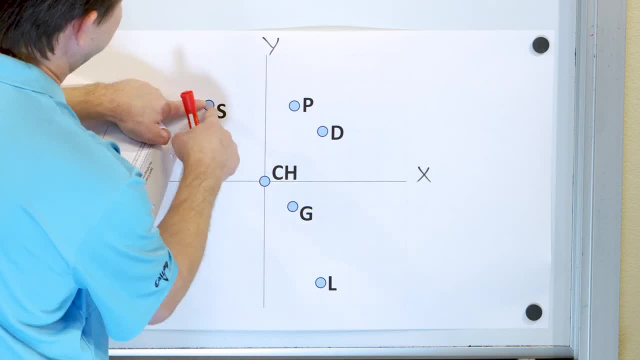 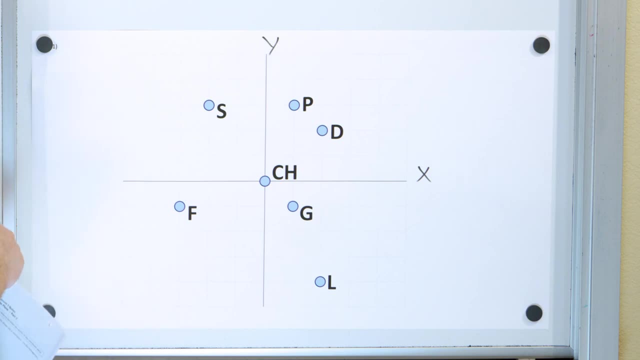 flying directly from the school to the grocery store. How far is that distance? Well, you really can't figure it out other than to calculate it or to measure it. If you got a ruler, I guess you could measure it. But we can calculate it because we can make a triangle out of this situation here. 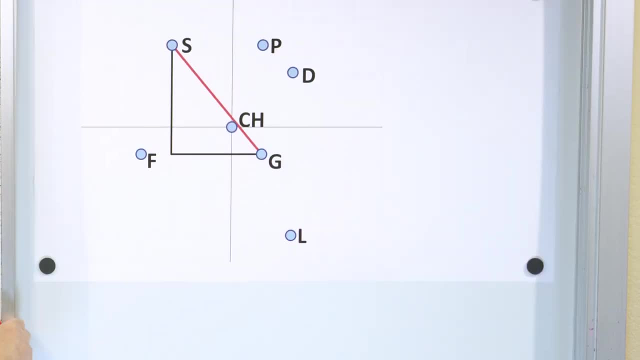 So let's go ahead and draw that triangle To make sure we understand: The school to the grocery store. this distance is what we're trying to find. And then these are the other two sides of the triangle. Now you might say I'm not given. 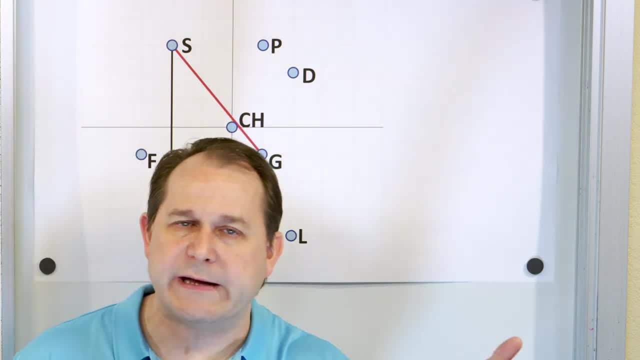 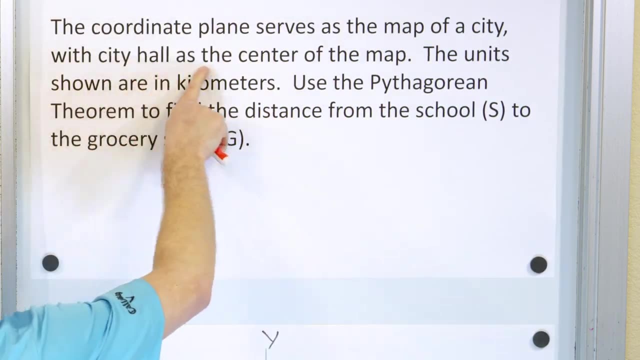 those distances, but you really are because everything is on a grid. So if you want to say that the or actually says in the problem statement it says city hall is the center. the units shown are in kilometers, right, So it might be like here's city hall and then this: 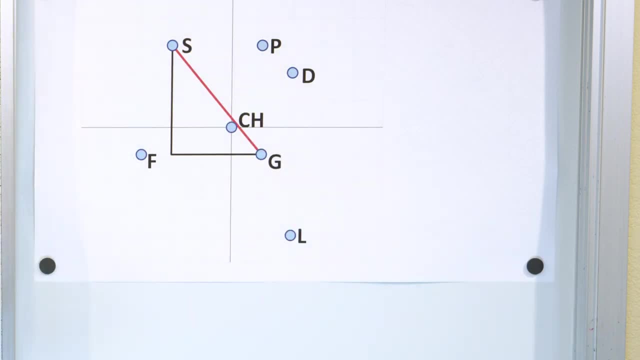 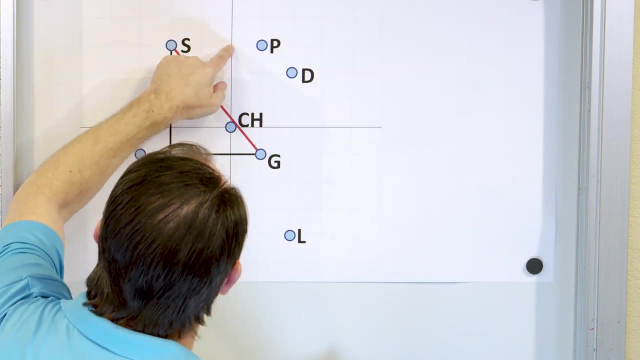 is west one kilometer east, one kilometer north, one kilometer south, something like this. Then the grid that you have would make sense, Or you might think of these being city blocks, So it'd be like one block, two blocks, three blocks up or whatever, whatever units you're dealing with. So how do we? 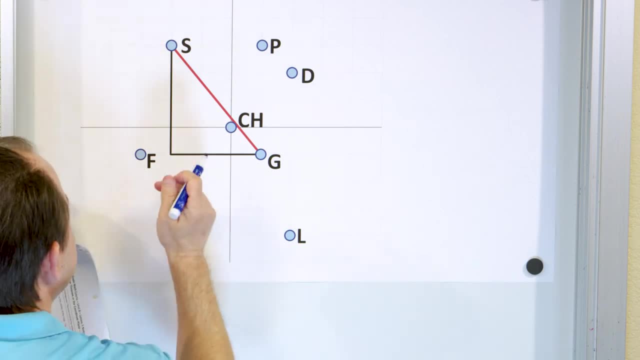 figure out what this is. Well, first of all, it's important for you to know that anytime you draw a triangle on a grid like this, you have a right angle in the corner, And so this is the hypotenuse, And we know that a squared plus b squared is equal to c. 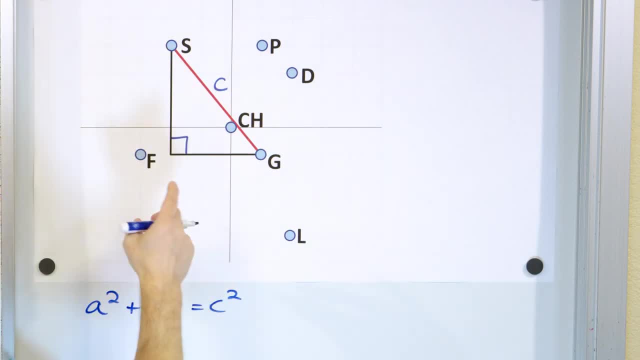 And we're going to call this a and b. What are the distances? Well, I just count them. I start here and I say I could put the points. I could put the x, y points if I wanted to, but I don't. 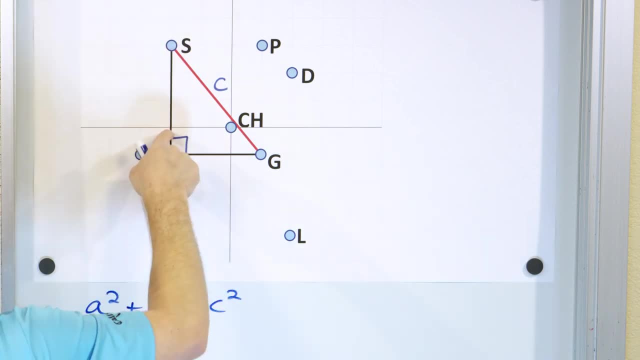 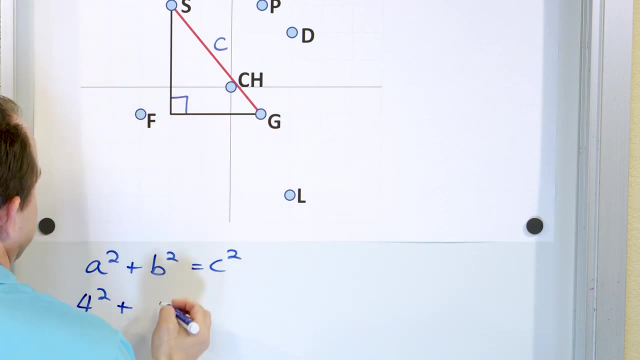 need to. I can just count one, two, three, four distance units down for a, so four squared. And then, starting here, one, two, three distance units in this direction, like this, And that has to equal c squared, because this is the other side of the triangle. And then I know that four times. 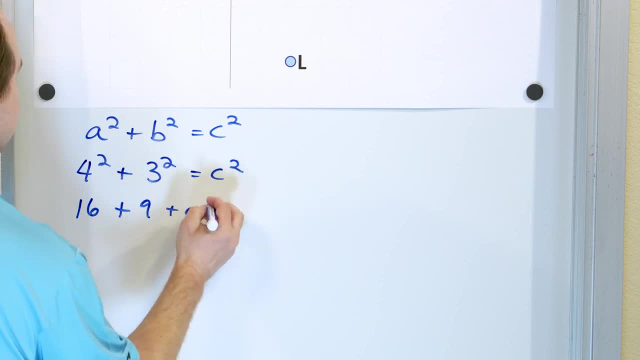 four is 16.. And I know that three times three is nine. And if I flip it around and put c squared here, then the 16 and the nine is 25.. And how do I get rid of this? Well, I say: c squared is equal to 25.. 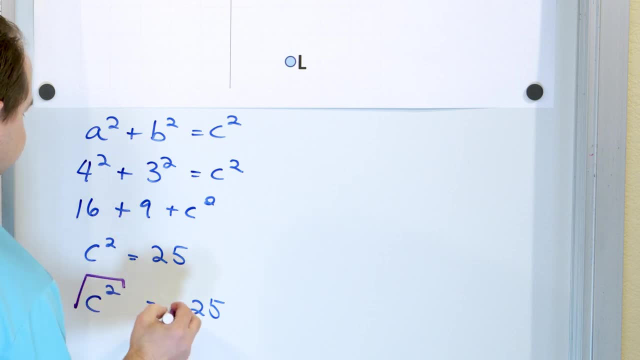 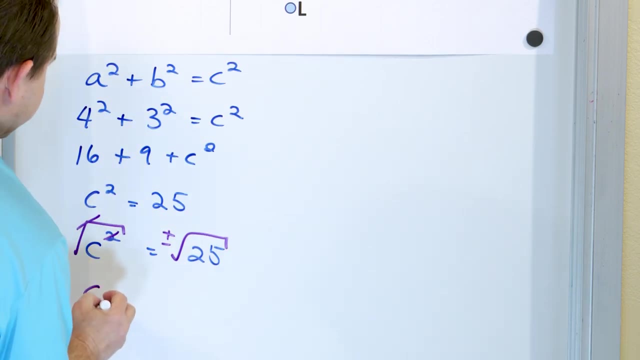 So if I want to get rid of this square, I have to do the opposite: the square root, And if I'm adding my own radical, I have to insert my own, plus or minus. The square root cancels with the square, leaving behind the distance c. 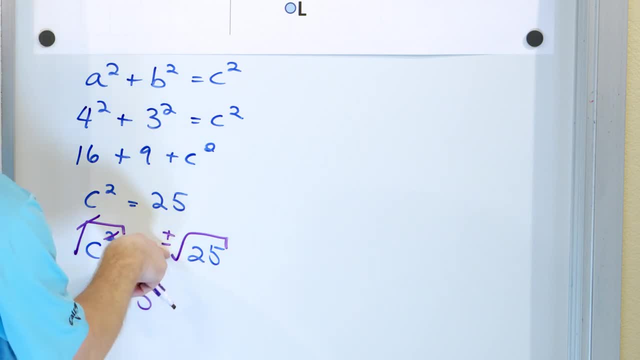 The square to 25 is five And of course there's no such thing as a negative distance. So I'm going to throw away the negative distance and say it's positive five. Now we said the distance units in this was measured in kilometers. So this is going to be five kilometers And that's an exact answer. 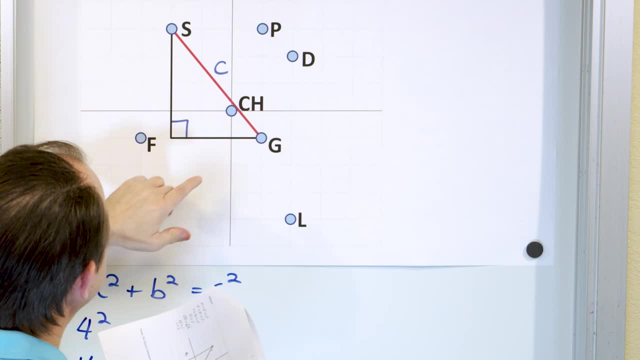 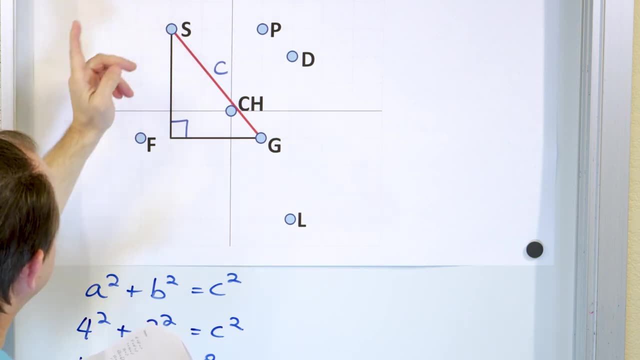 So what this means is that if the map were laid out the way it is, so that City Hall were in the center right, And then if you could go like two kilometers to the west and then three kilometers north to get to the grocery store right, And then from City Hall one kilometer to the east. 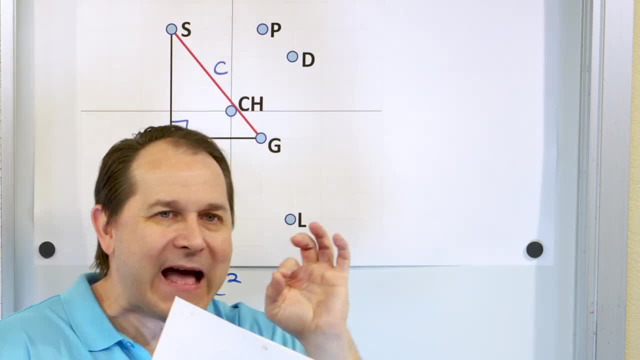 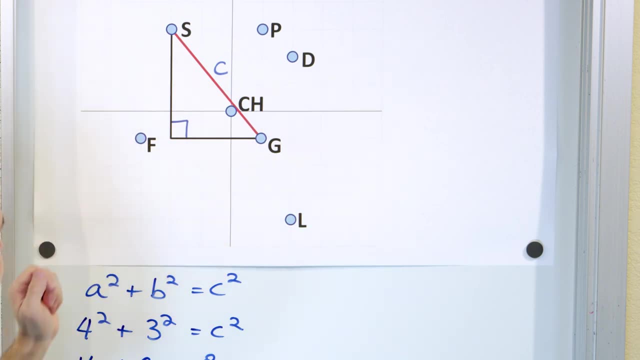 to the right and one kilometer down was the grocery store. If that grid system was how you defined it in terms of kilometers, then the straight line distance from here to here is given by the Pythagorean theorem and works out to be exactly five. 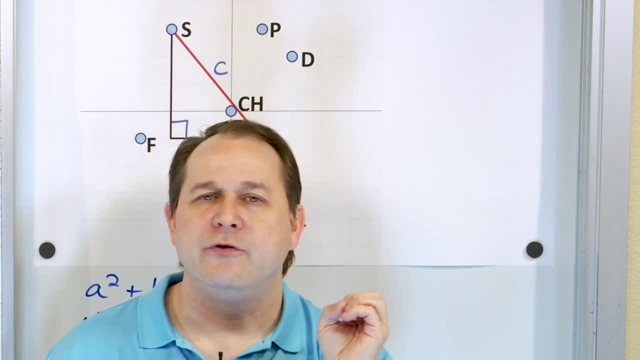 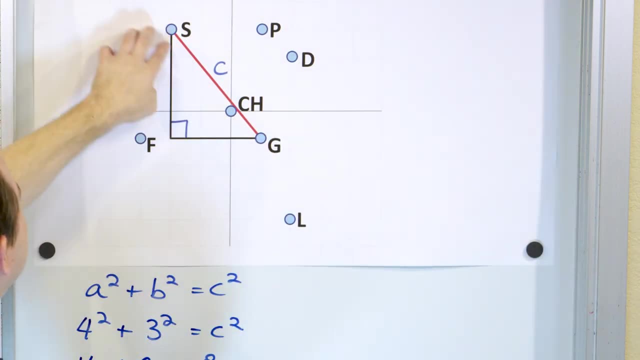 kilometers. Now this makes sense because, remember, one of the special triangles for the Pythagorean theorem is three, four, five, right? So you have three, four and then five. So we probably could have guessed before calculating. but it's good to do the full. 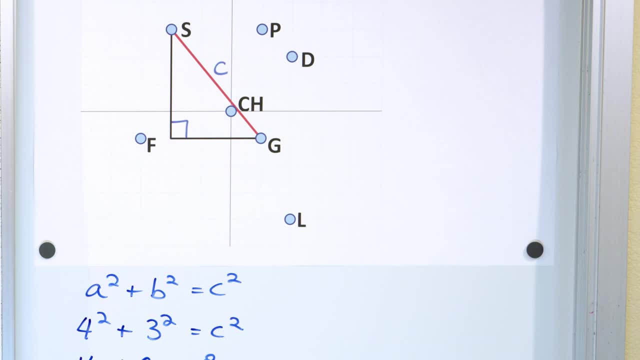 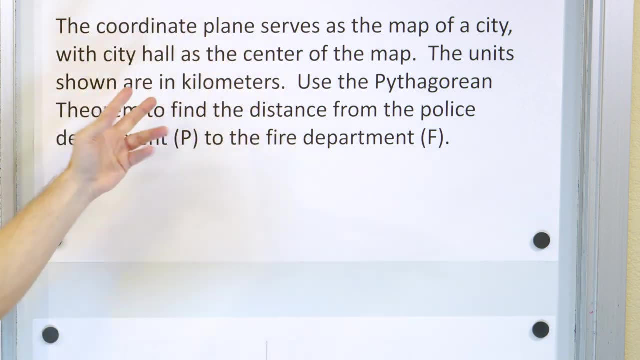 calculation. All right, let's take this one down and do our next problem. All right, problem number one: we're going to find the coordinate plane map of the city, kilometers, all that stuff is the same. We're going to find the distance between the police department P and the fire department F. 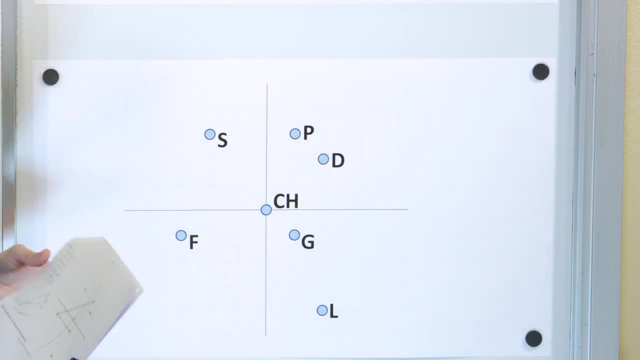 So P to F. So P is right here and F is right here. So we have to figure out some kind of right triangle. Now there are multiple triangles. I could draw one like this if I wish, or I could go the other direction like this: It's going to give the same answer. So let's just draw between. 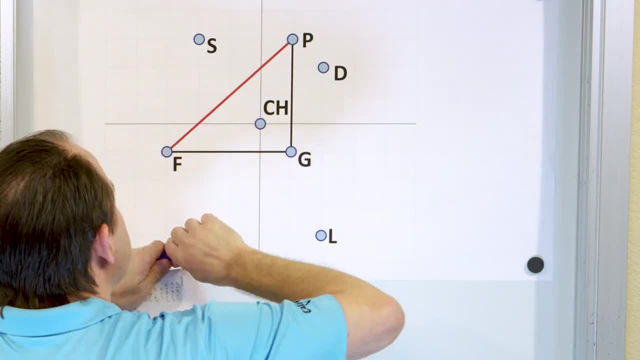 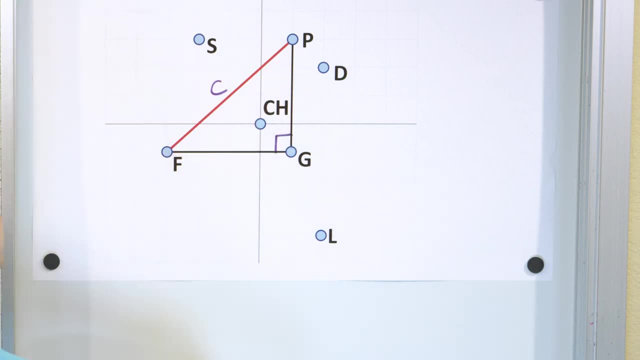 P and F, the triangle that makes the most sense like this. Notice, it's always a right triangle on a grid like this. So here we have the hypotenuse C. That's what we're trying to find in red. These other two sides will be A and B. I could put the coordinates of the points, but it doesn't. 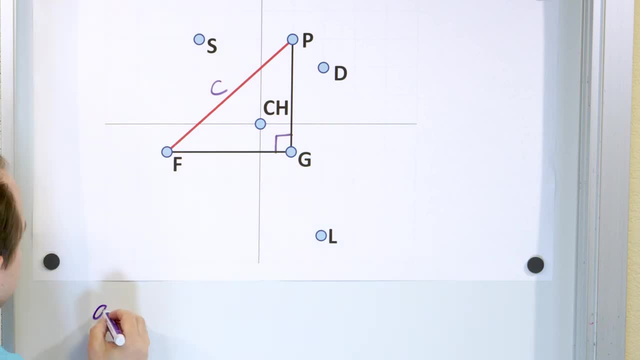 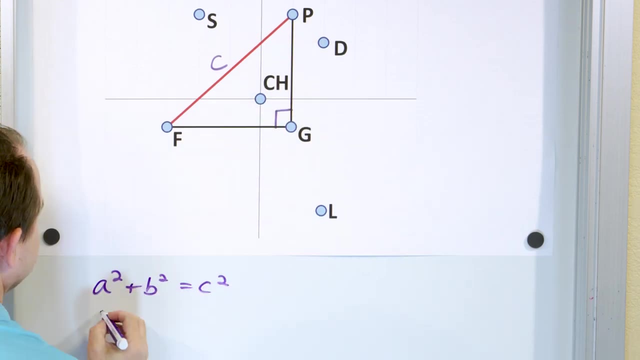 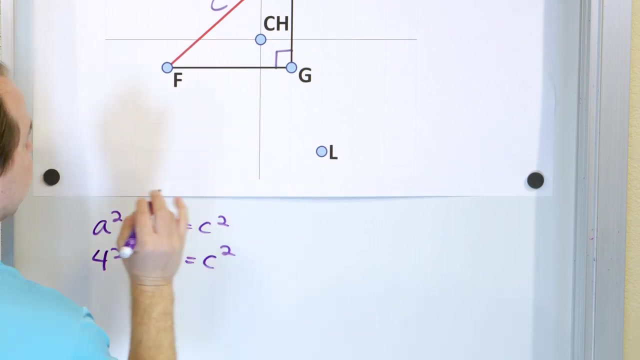 matter. I can just count them right off of the page here. So we know that A squared plus B squared has to equal C squared. And A and B are these sides one, two, three, four, So four squared- plus B, one, two, three, four, So four squared. And C is what I'm trying to find. So I put C. 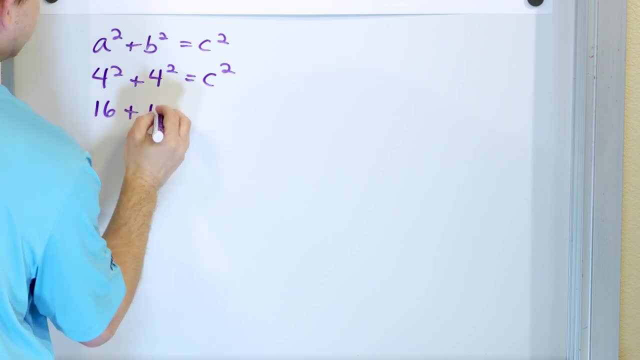 squared right there. So here I have 16.. And then I have 16. And when I flip this around I get C squared is equal to 32.. So I need to solve this. C squared is 32.. Now how do I get rid of that square On the C? I have to do the opposite. 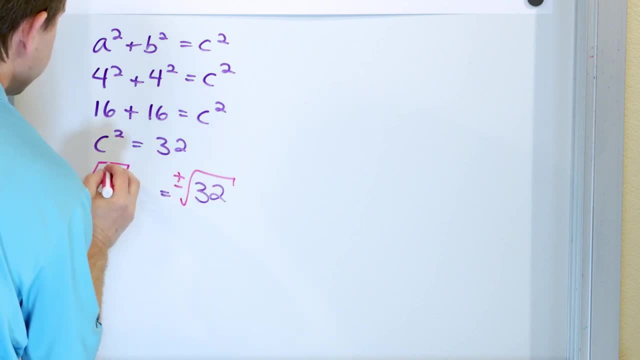 square root. So I have to take the square root and add that plus or minus N, Cancellation will happen And the distant C will be whatever the square root of 32 is. Now how do we figure out what that is? That's the trick, right? So I don't know what that is. That's not a perfect square. 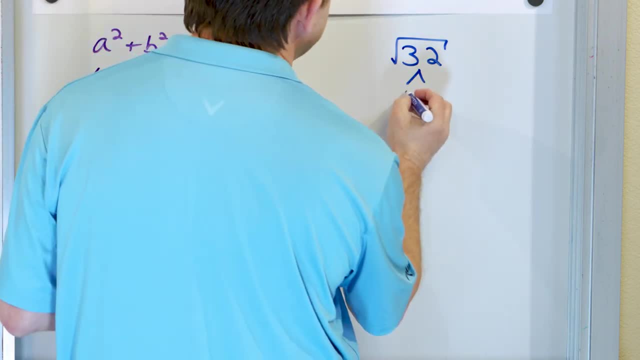 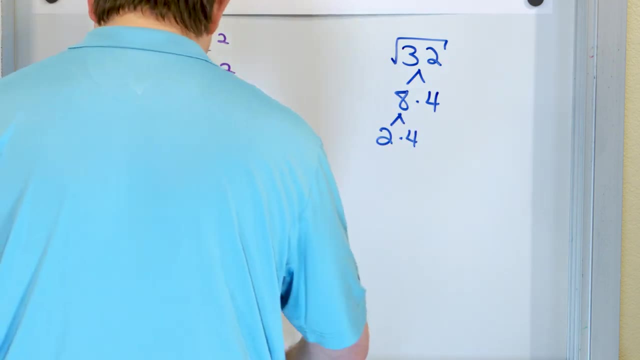 So you need to break it into something simpler. So I know that 8 times 4 is 32.. And I know that 8 is 2 times 4.. Now I can break these 4s apart, but it won't change anything. I'll still get the same answer, because I see a pair of 4s. 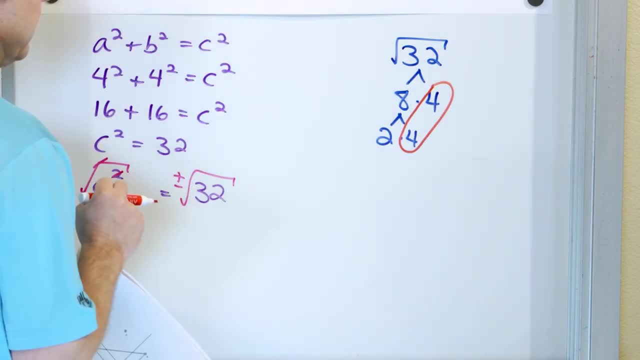 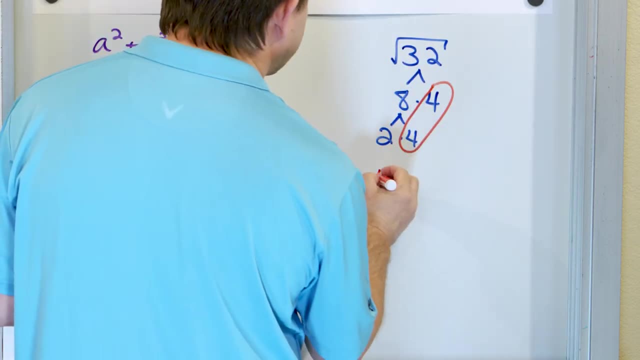 and I can immediately circle any pair I see in the bottom of the tree. If I break these apart into 2s and pull out those 2s and multiply them, I'm going to get the same thing. So a single 4 will come outside and the square root of 2 will be left behind. So I'll have 4 times the square. 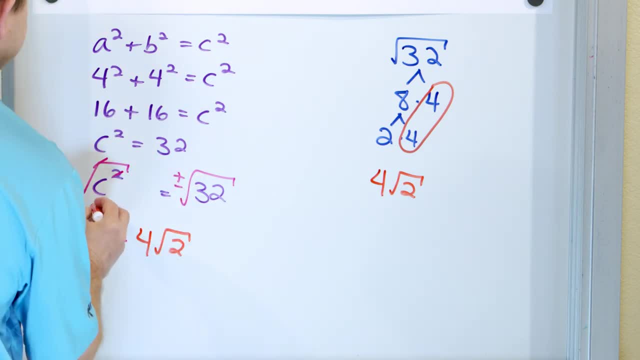 root of 2.. We're going to throw away the negative answer. It doesn't make sense, And so the answer is 4 times the square root of 2.. Now if you take the square root of 2 and put it in the calculator, 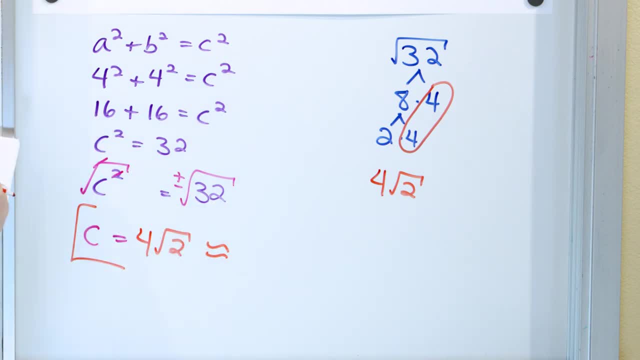 and you get 1.41,. multiply that by 4, you'll get 5.66, roughly kilometers. Of course you have to round it. If you put 32 in the calculator and take the square root, you'll get the same thing. So these two are just different ways of writing the same thing. 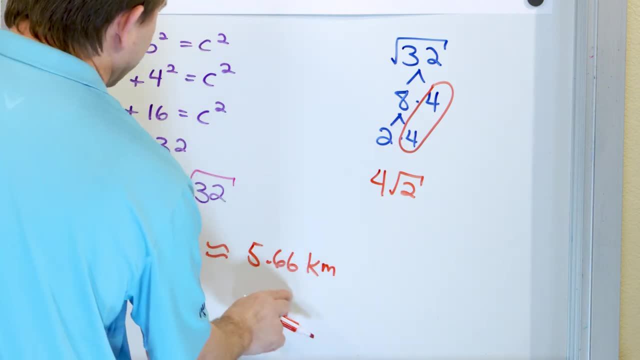 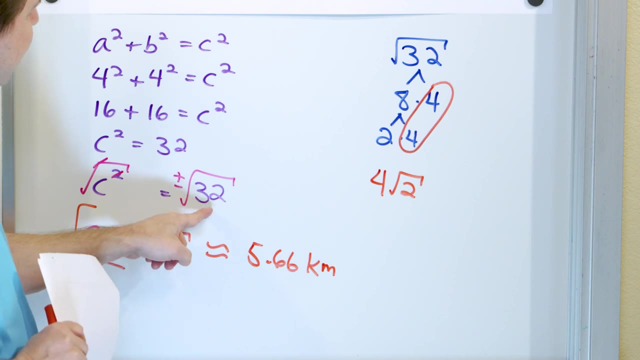 4 times the square root of 2, and you're talking about kilometers here, or roughly 5.66.. Kilometers. Now, this also makes sense, because we know that 5 times 5 is 25, and we know that 6. 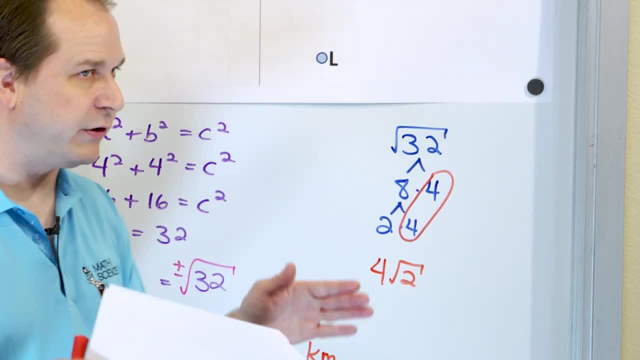 times 6 is 36.. So since we're trying to find the square root of 32,, which is right in the middle of that range, it makes sense that the answer would be between 5 and 6, which is what we found. 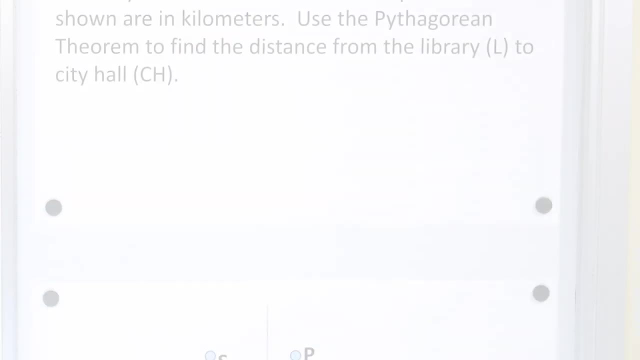 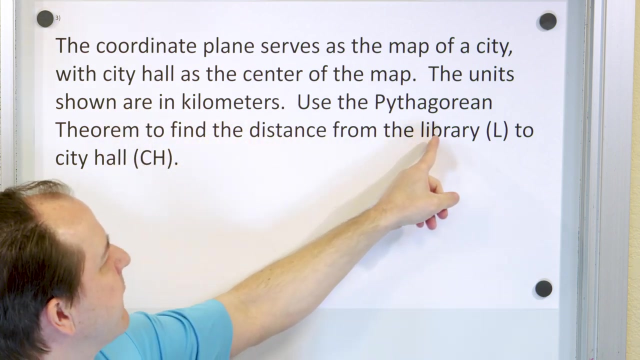 Let me take this down and we'll do our next problem. All right, here is our last problem. Same story with the kilometers and the map. We're going to use the Pythagorean theorem to find the distance from the library L to the city hall. So the library is here, The city. 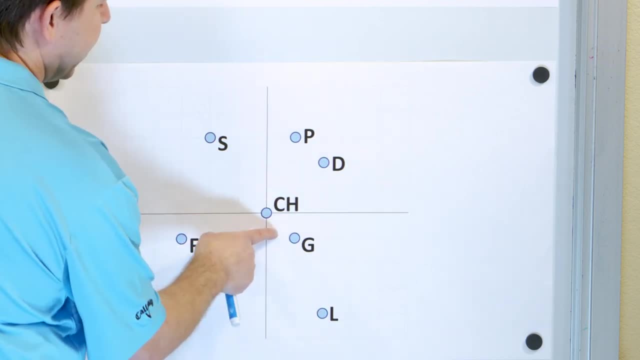 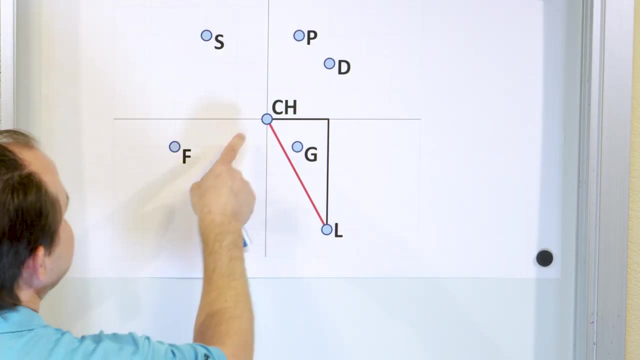 hall is here, The city hall is at the very center of town and the library is diagonally down this direction. So let's draw a picture of what we're trying to actually find. We're trying to find this distance here, so we're going to form a triangle out of it And of course, this is a 90-degree. 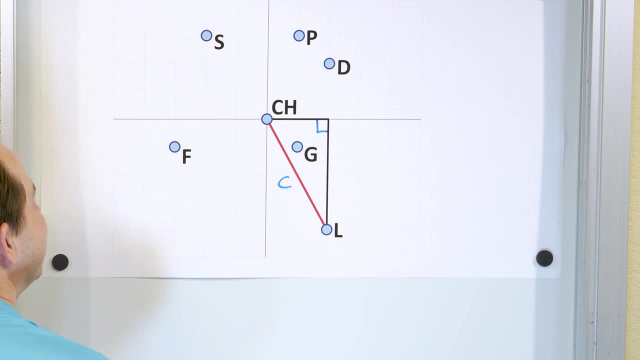 angle, so it's a right triangle, And so that means this is the hypotenuse C, And we can then write that C squared is equal to A squared plus B squared. Now usually I say A squared plus B squared equals C squared, but you know you can flip things around, So we're going to do a. 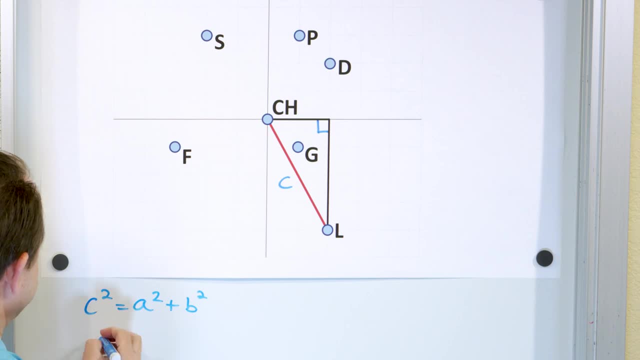 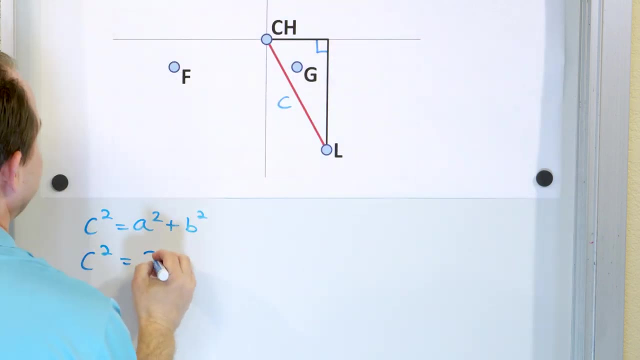 round. We're just going to write it like this from now on, since we're solving for the distance C, So C squared is A, which is one side of the triangle. This is one, two distance units, two kilometers, So two squared. And then this is one, two, three, four, So four squared. So what? 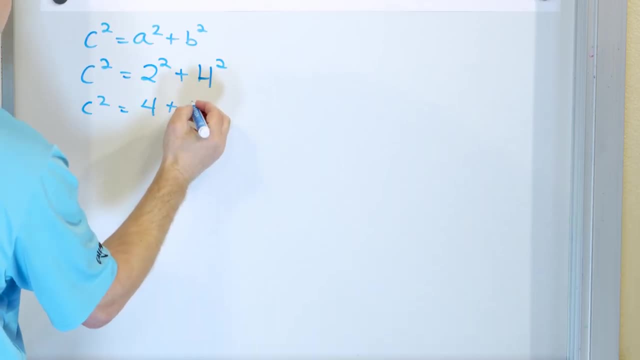 do we have here? Two times two is four, and four times four is 16.. And so C squared is going to be equal to 20.. Now we don't want C squared, We want to figure out what C is equal to. 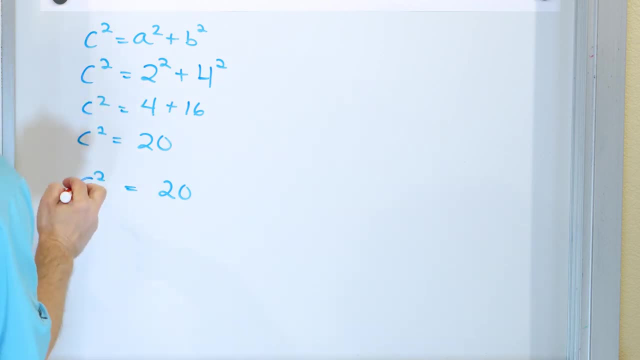 So how do we do that? We have to do the opposite of whatever we've done here, which is squaring. So we're going to do the square root and we're going to do it to both sides, and we have to add the 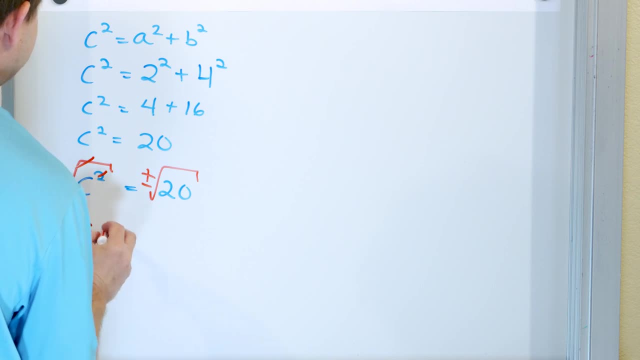 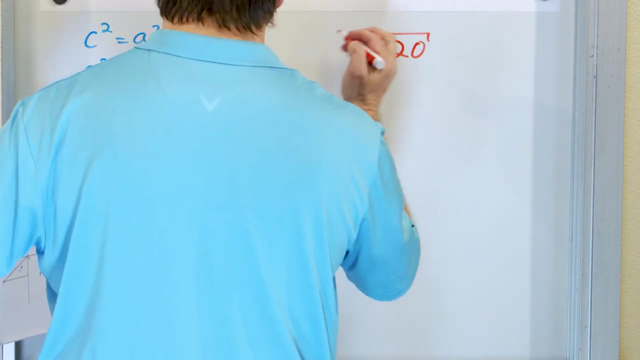 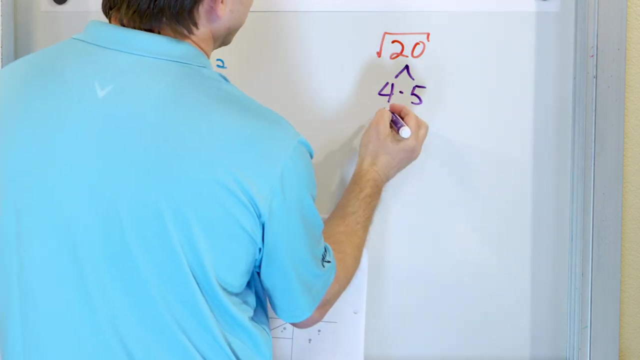 plus minus. So we're left with: C is equal to. we're going to throw away the negative answer. We're going to get the positive answer: square root of 20.. How do we take the square root of 20?? Well, we can write this as: four times five is 20.. The four we can write is two times two. 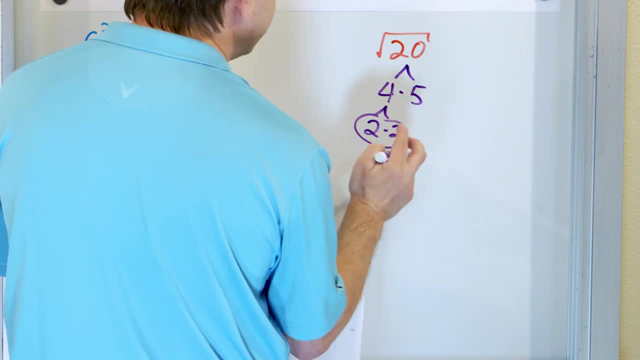 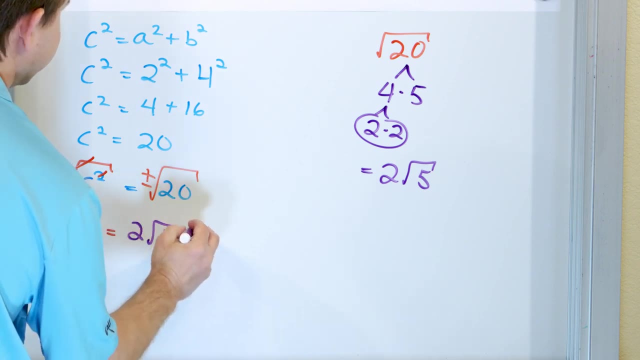 and we have a positive answer. So we're going to do the square root of 20.. So we have a pair right here. So it comes out as the single two comes out, square root of five is left behind. So we have two times the square root of five and the units here were all in.